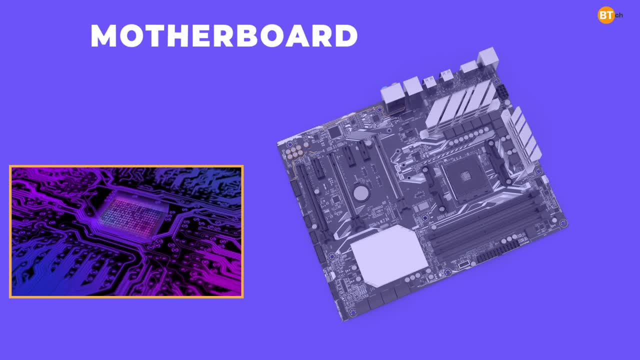 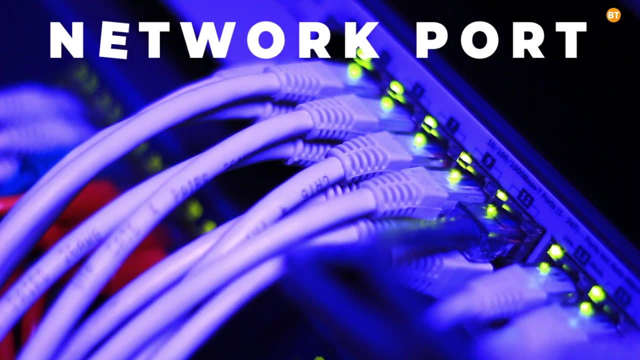 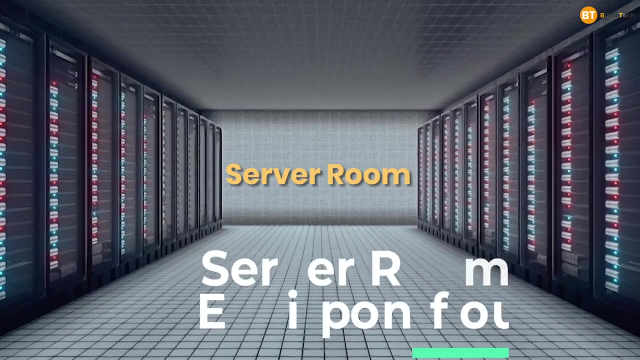 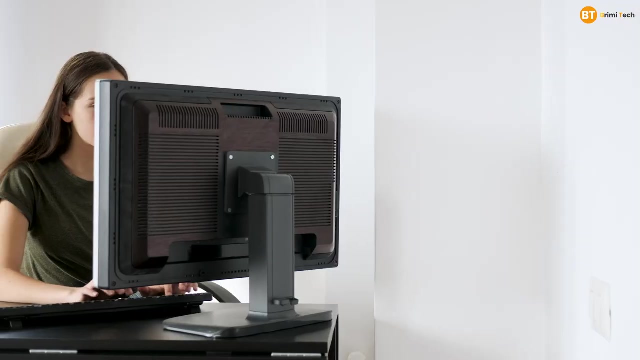 What are the main components of a server: Motherboard, CPU, Memory, Hard drive, Network connection, Power supply, Etc. Server Room Environment and Requirements. The server needs to be installed in an exclusive environment. You can use your desktop computer in your bedroom. However, a server needs a server room. 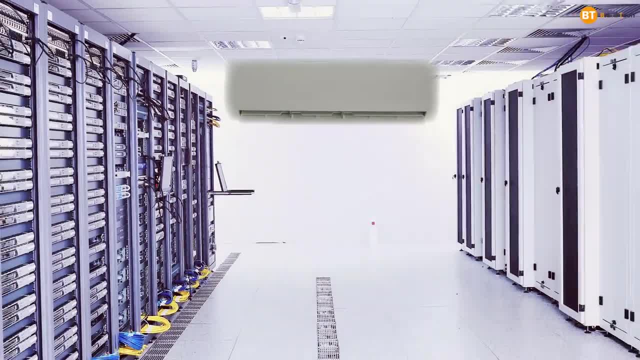 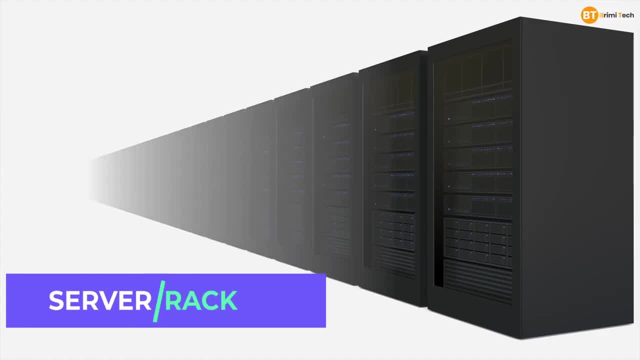 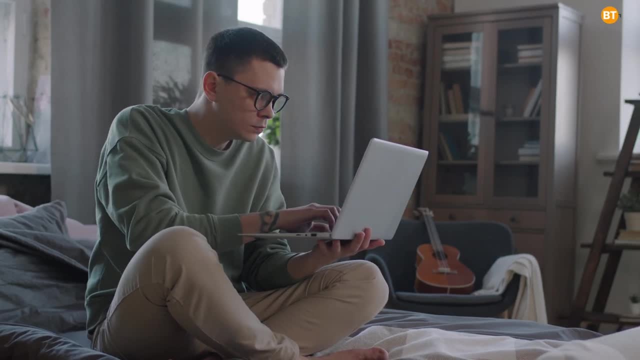 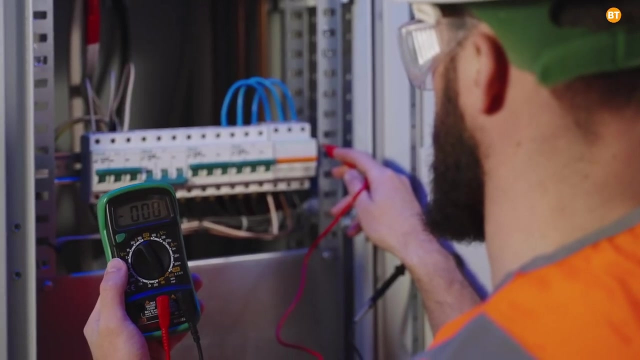 A server room is always kept clean and tidy. The room should be air-conditioned. The server is placed in the server rack, where multiple servers can be placed in a single rack, but a desktop computer can be placed anywhere in the room. A server needs a robust power supply system so that electricity can be supplied uninterruptedly. 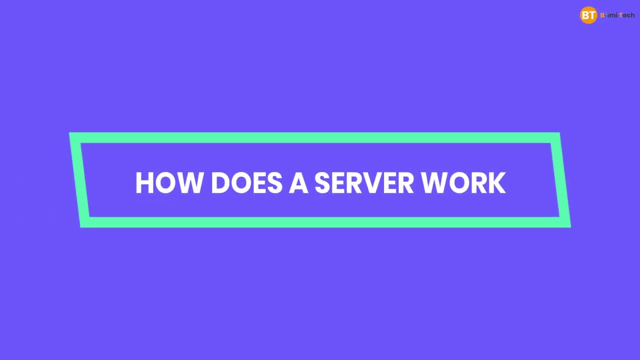 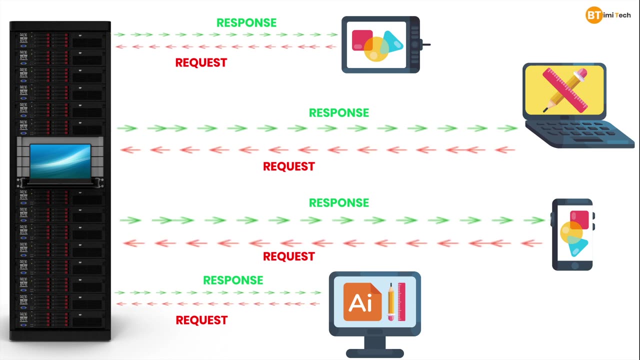 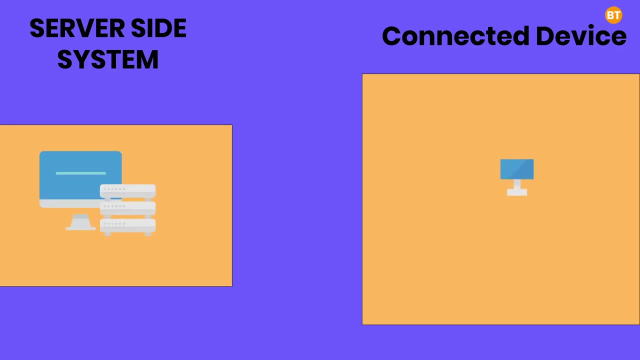 How does a server work? To act as a server, the computer system should be able to receive the request for a service. A server can send a request from the client via a network connection. When a client needs functionality or information from a relevant server, it sends a request via a connected network. 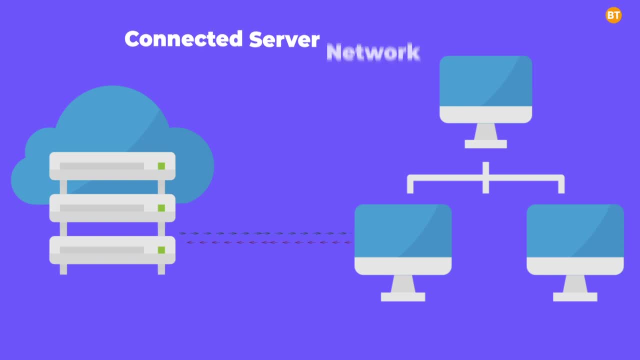 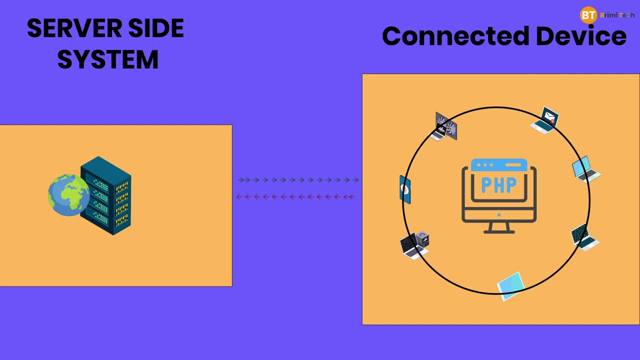 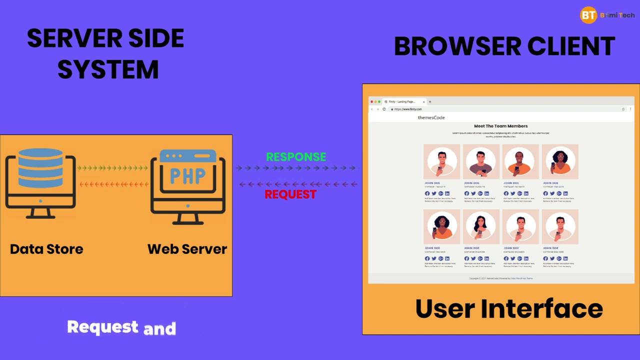 Upon receiving this request, the server provides the requested information. That's how a client and a server can communicate with each other. This process is called the request and response model, as well as the call and response model. In most cases, a server has to perform multiple tasks. 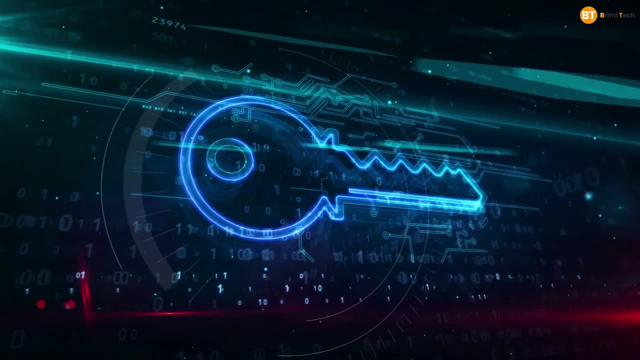 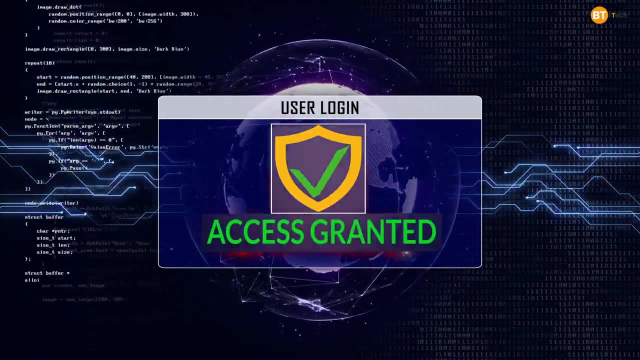 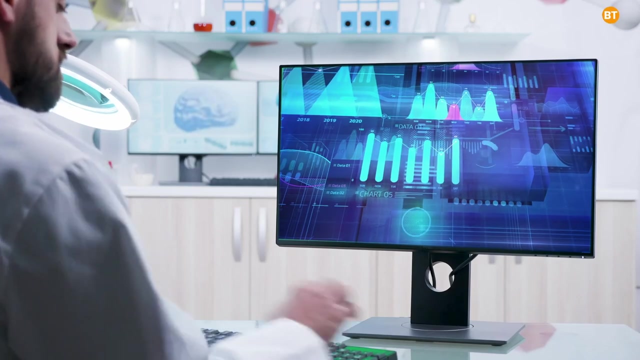 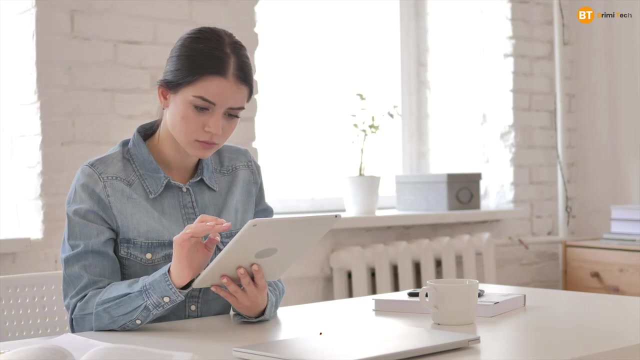 On a single request and response, such as identification of the request sender, make sure that the requested client is authenticated to access the data and return the desired result in a specific way. Now we will explain to you how a server works in detail. Whenever you browse the Internet, you access a web server. 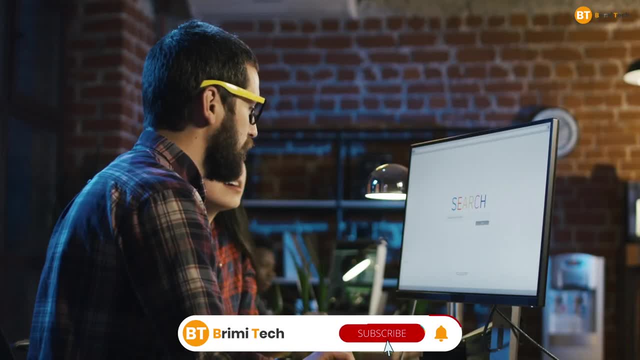 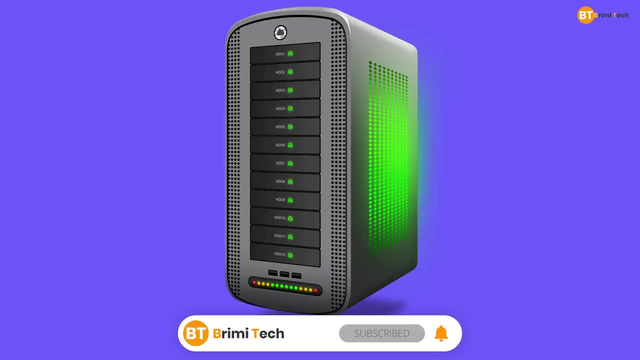 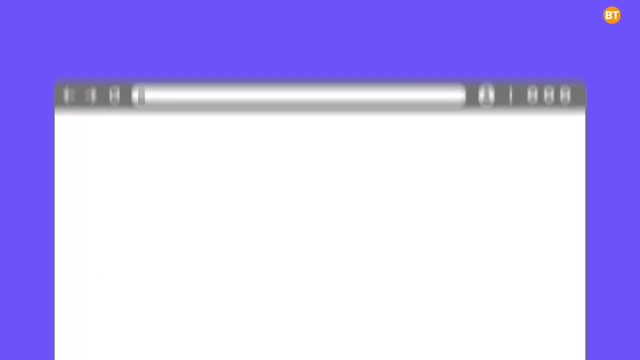 When you type a URL on the address bar into a web browser like Google Chrome, Mozilla Firefox, your computer communicates with the hosting server and grabs the information onto your computer. Let's simplify the steps. Open Google Chrome browser. Enter URL on the address bar. 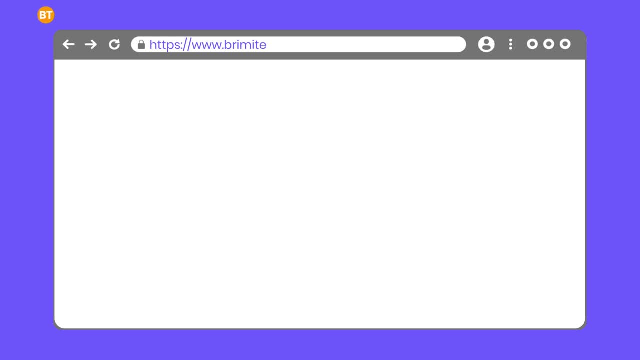 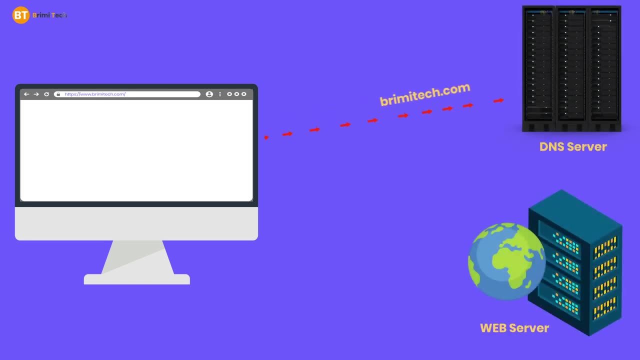 https colon slash slash www dot brimatech dot com. The browser features the IP address of the brimatech dot com domain from the DNS server. Chrome sends HTTP requests to the server at that IP address. HTTP server accepts the request, looks for the requested document and sends it back to the browser. 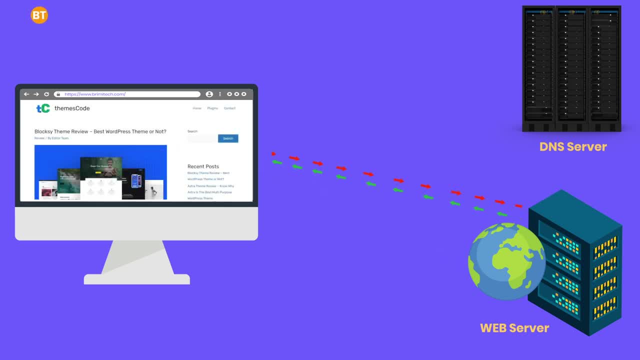 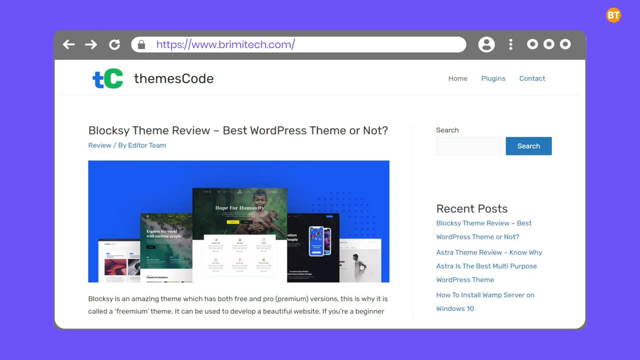 Browser receives the HTTP response from the server and generates all of the data. Browser generates all of the data required to show the website. Finally, Google Chrome browser displays the website on your device's screen. This is how a web server works. Pretty simple, isn't it? 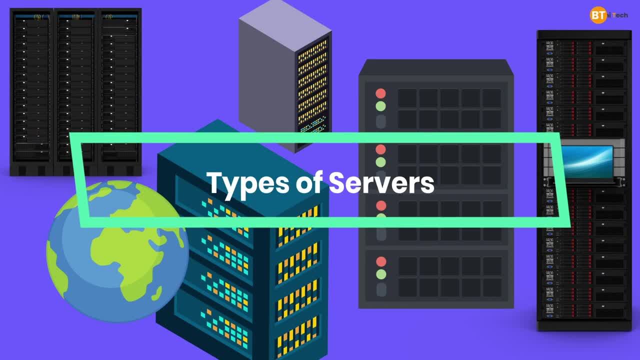 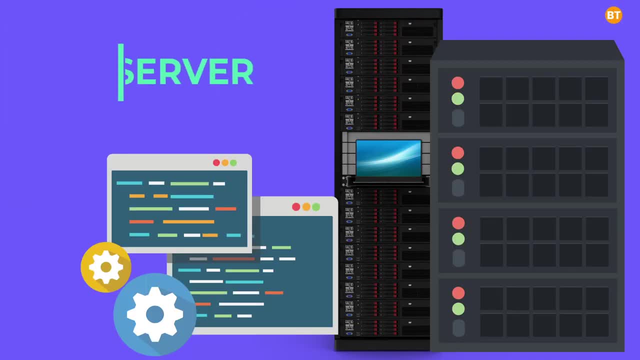 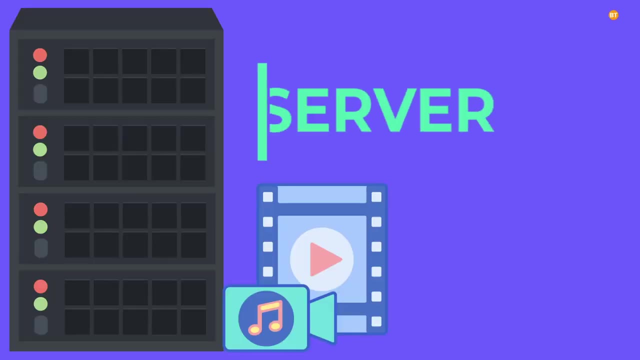 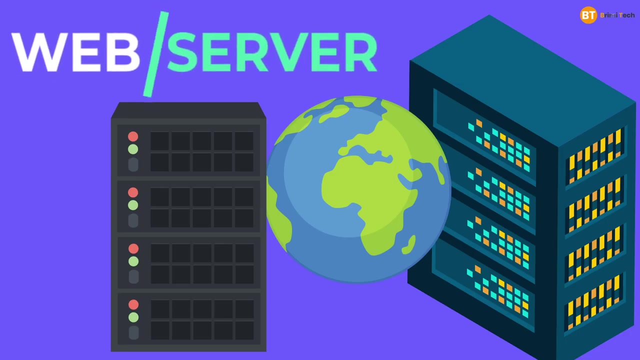 Types of Servers. A wide variety of servers are used to accomplish a variety of tasks, including Database Server, Application Server, Fax Server, File Server, Mail Server, Digital Server, Game Server, Media Server, Print Server, VPS Server, Virtual Server, Web Server, Etc. Desktop Computers vs Servers. 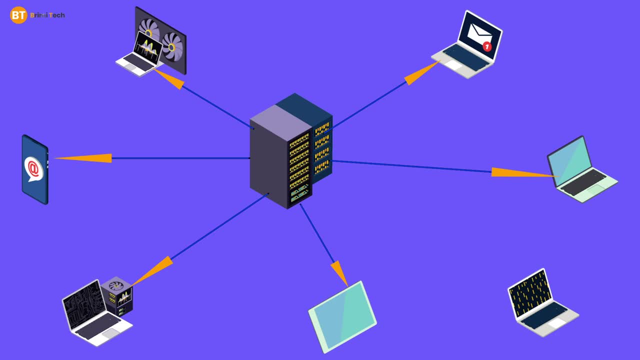 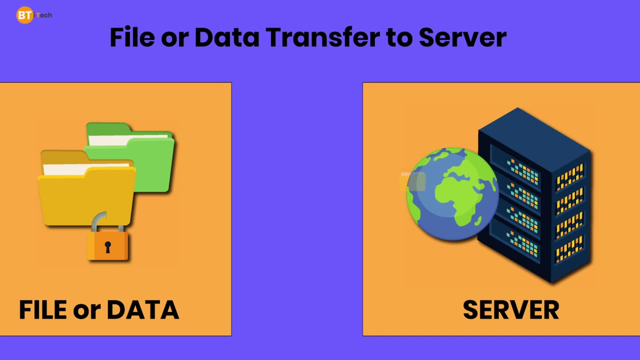 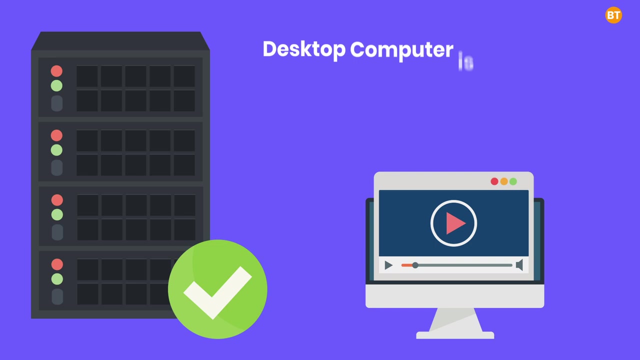 Many desktop computers can be connected to one single server. Server machines can store a huge number of files, including data and applications, than a desktop computer's. A desktop computer is smaller than a server computer. The desktop computer needs access to the server computer to do some particular tasks. 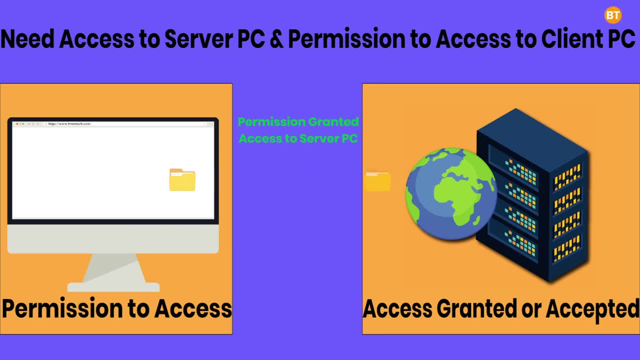 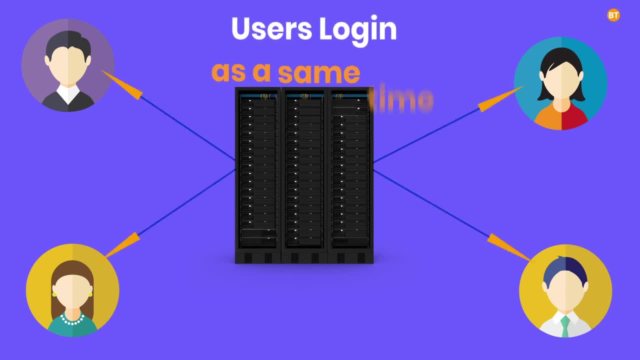 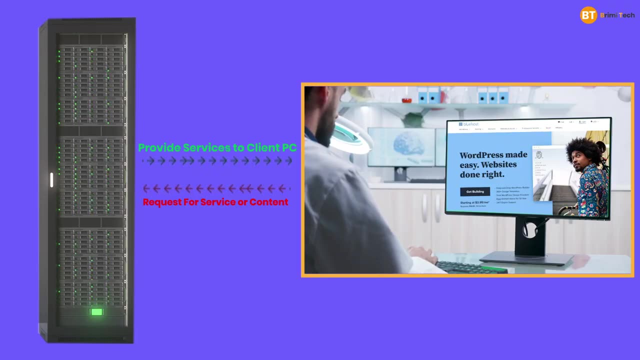 The server computer gives access to the desktop computer and serves the purposes of the clients. A server allows several users to log in at the same time, but a desktop computer only allows one person to log in at a time. Desktop computers request the server computer for service or content. 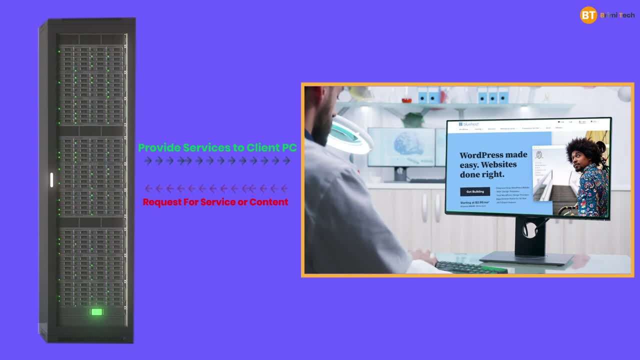 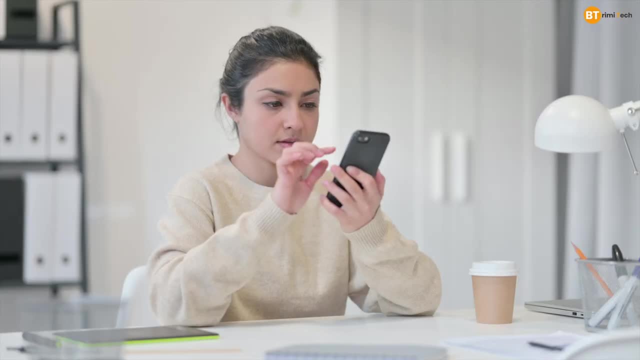 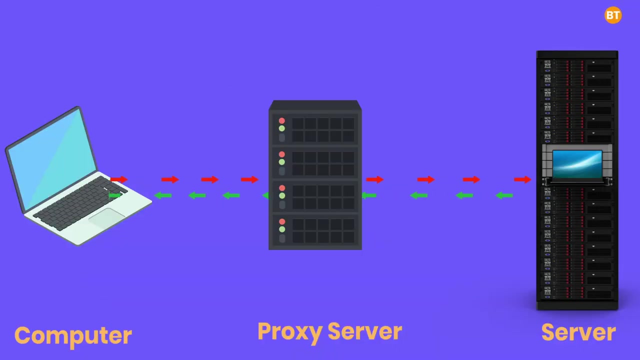 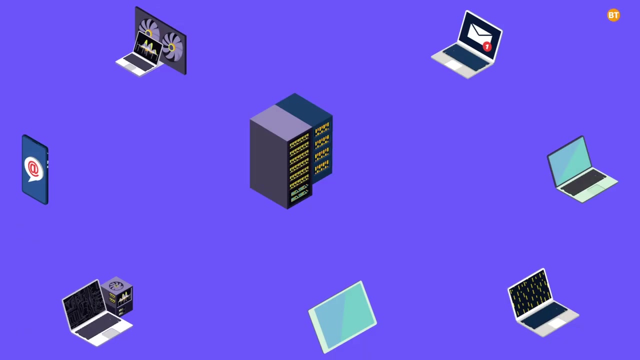 Server computers usually provide services based on desktop computers' requests. Example of Client Computers, Notebook, Desktop, Smartphones, Etc. Example of Server: VPS Server, Application Server, Proxy Server, Mail Server, Database Server, Etc. Now let's observe the differences more deeply in terms of technology.